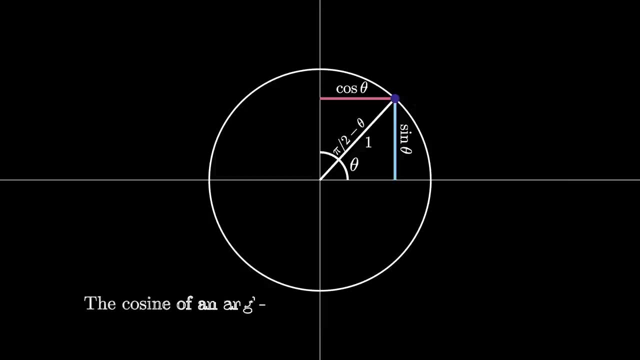 to theta is pi over 2 minus theta. so the cosine of theta is really the sine of the complementary angle. That means that the cosine of theta is equal to the sine of pi over 2 minus theta. Now draw the line that is tangent to the circle at the point and perpendicular to the. 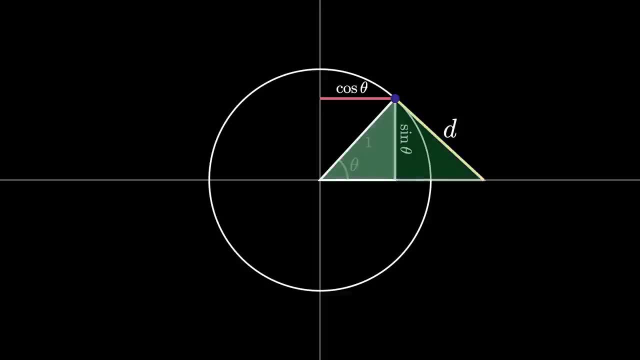 radius. Let's label the line segment D, Because these two pictured triangles are similar. that means that the ratios of the side lengths are equal, so that D over 1 is equal to the sine of theta divided by cosine of theta. Therefore, the length of this new line segment must be the sine. 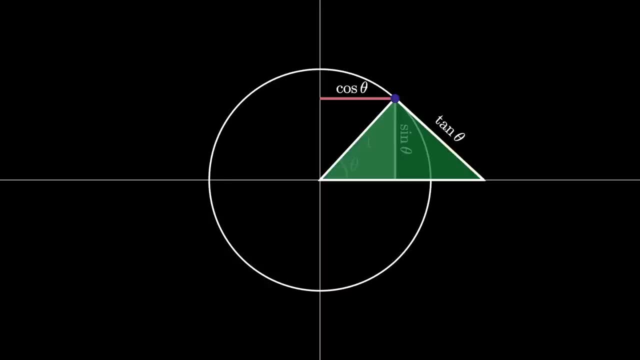 of theta over cosine theta, which we call the tangent of theta. We can use the same triangle similarity to compute the length of the hypotenuse of this new triangle to be 1 divided by the cosine of theta, which we then call the secant of theta. Now we perform a similar process, starting at the. 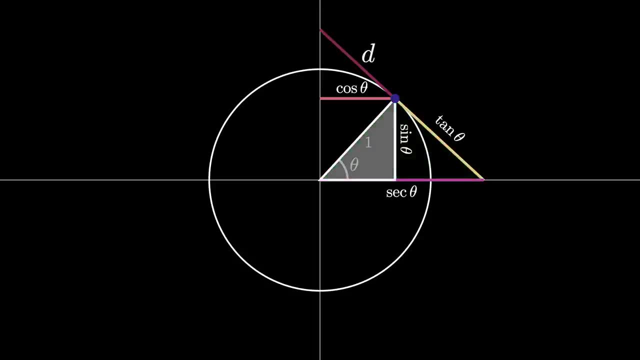 point on the circle and drawing a line perpendicular to the radius that connects to the y-axis with a length of D. Because the two pictured triangles are similar, we can see that D divided by 1 must equal cosine of theta divided by sine of theta. Therefore, the length of the new line we drew must be cosine of. 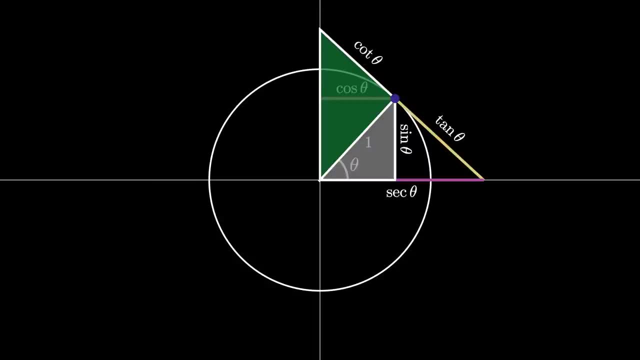 theta divided by sine of theta, and we define this to be the cotangent of theta. Similarly, we can compute the length of the hypotenuse of this new triangle using the similarity of triangles to be: 1 divided by the sine of theta, which we define to be the cosecant of theta. 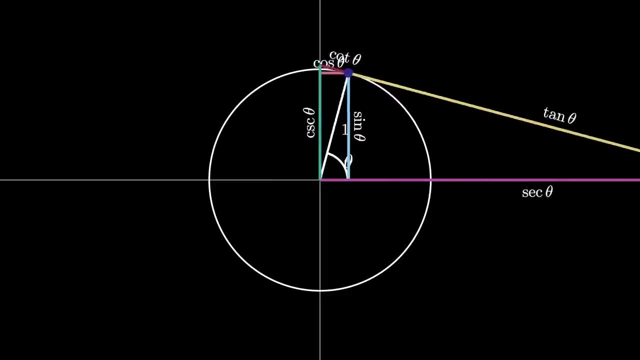 As we change the angle, theta, we see that all of these values change as well. In fact, if we let theta be pi over two, we see that tangent and secant are undefined at this point because those two lines don't intersect along the x-axis. Likewise, if we let theta vary all the way down to zero, we see a similar fact. 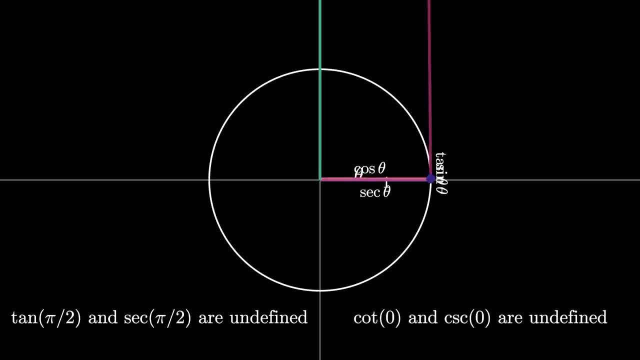 about the cosecant and the cotangent of zero. They are both undefined as well. We can get even more information from this diagram as we let theta vary. We see in particular that the sine function and the cosine function outputs must be between negative one and one. 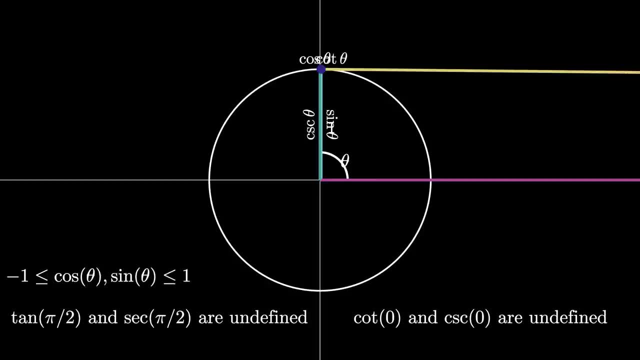 as those lengths can't extend outside the unit circle, which has a radius of one. And likewise, we see that the cosecant and the secant have absolute values that are greater than or equal to one. And finally, we see that the tangent and the cotangent can take on any 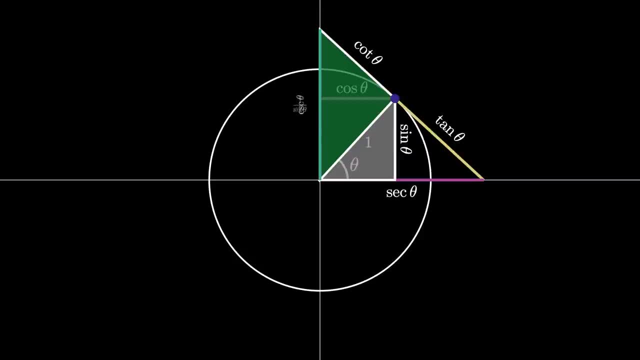 the similarity of triangles to be 1 divided by the sine of theta, which we define to be the cosecant of theta. As we change the angle theta, we see that all of these values change as well. In fact, if we let theta be pi over 2, we see that tangent and secant are undefined at this point. 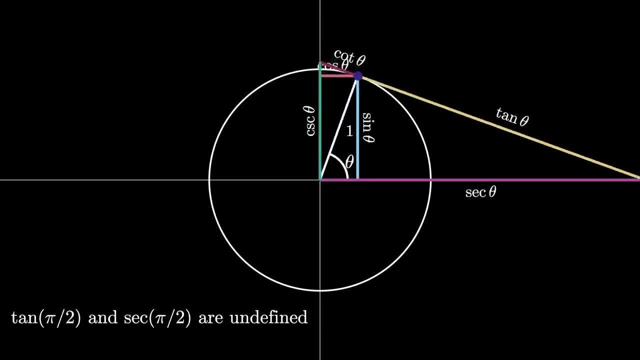 because those two lines don't intersect along the x axis. Likewise, if we let theta vary all the way down to 0, we see a similar fact about the cosecant and cotangent of 0,. they are both undefined as well. We can get even more information from this diagram as we let. 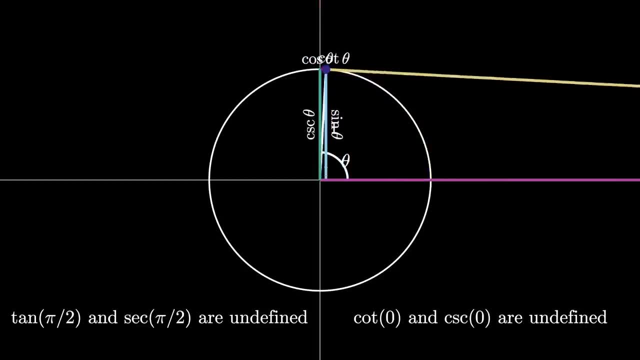 theta vary. We see, in particular, that the sine function and the cosine function outputs must be between negative 1 and 1, as those lengths can't extend outside the unit circle which has a radius of 1.. And likewise we see that the cosecant and the secant have absolute values. 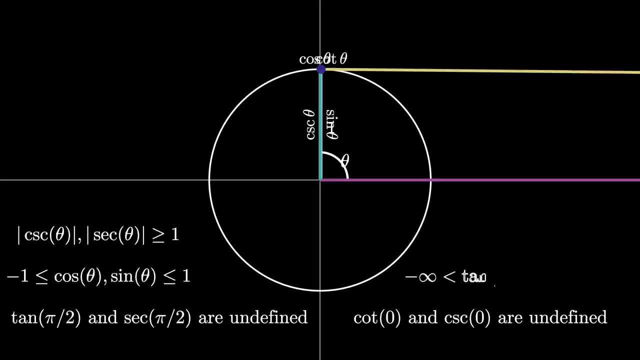 that are greater than or equal to 1.. And finally, we see that the tangent and the cotangent can take on any value between negative infinity and infinity as we rotate around the circle. Returning to our general diagram, we can apply the Pythagorean theorem to gain more insight about 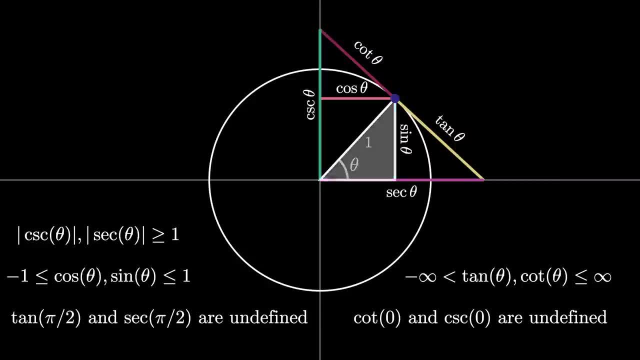 the trig functions. From this original right triangle we see that the sine squared of theta plus the cosine squared of theta must equal 1.. From the right triangle created by the tangent and secant values, we get that 1 plus the tangent squared of theta must equal the secant squared of. 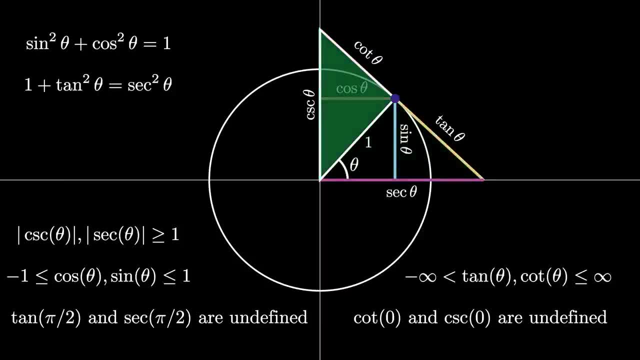 theta and from the right triangle, from the cotangent and cosecant values, we see that 1 plus the cotangent squared of theta equals the sine squared of theta. It's interesting to note that all three of these identities are really just the same, since they all 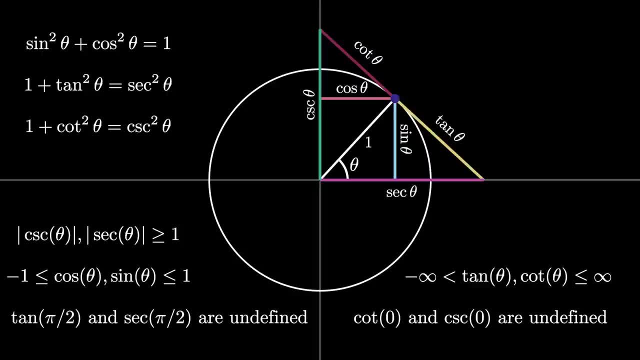 come from triangle similarity. Also, notice that these two triangles pictured here really contain the same information. it's just one contains the information about the complementary angle. Those values are simply the sine secant and tangent of the complementary angle. The prefix co-attached to all those words stands for complementary.